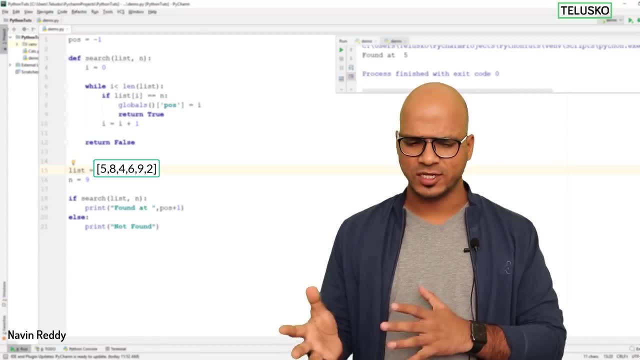 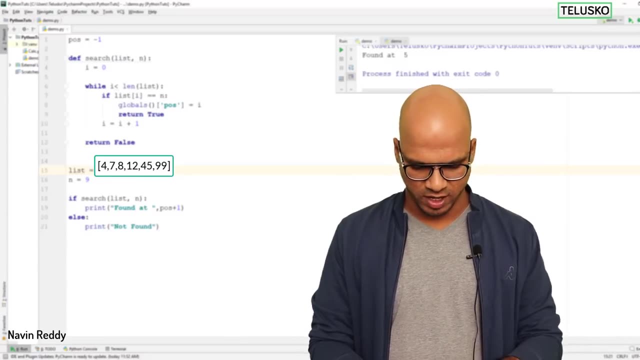 initial values. example. we are putting values like this right, So we will change it. We will have a value which is sorted right. So let's say 4, 7,, 8,, 12,, 45,, 99.. So let's: 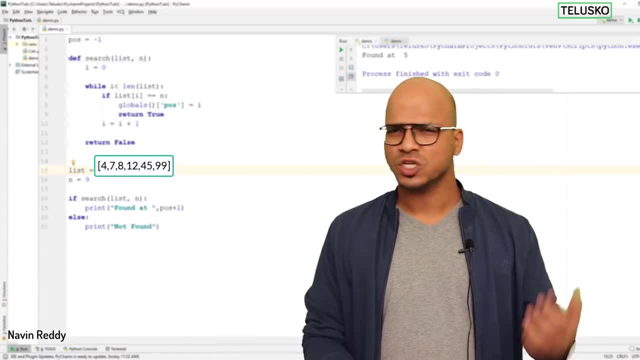 say we have this value, So we have six values. I want to search for a particular value, So instead of going for a linear search here, we will go for binary search. Now how that works. So let's imagine we have a list here, right? 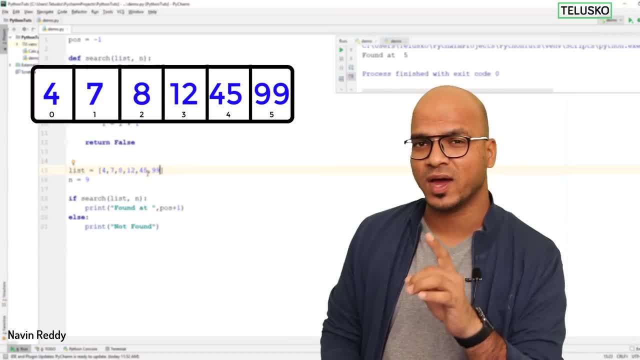 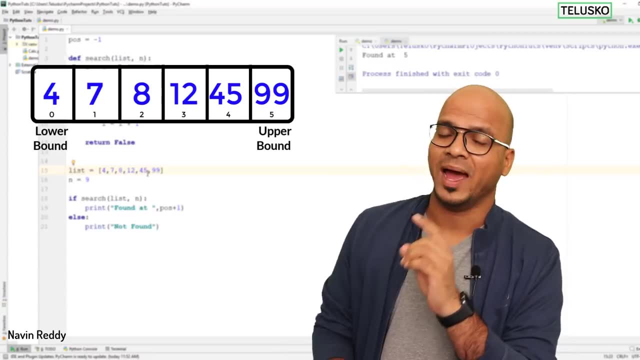 if you want to search for the element, what you will do is you will first specify the lower bound and the upper bound. okay, so, as you can see, the first value is a lower bound here. so the first value itself is a lower bound and the last value is the upper bound. you can say first or last, but 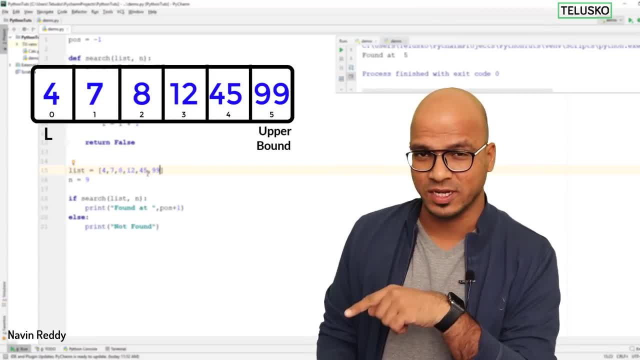 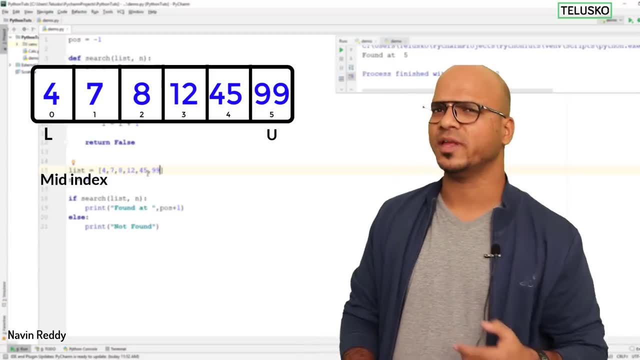 then let's go with this word l or u, so l is the first index and u is the last index. once you have assigned this thing, the next step you have to do is you have to find a mid index. now, how do you find a mid index? as name suggests, mid, it should be a midpoint of this lower and upper right. so 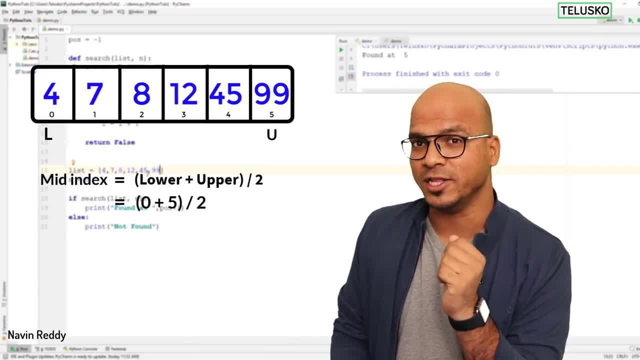 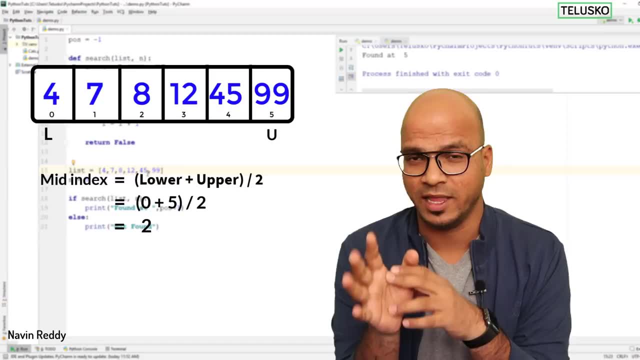 you will simply say lower plus upper divided by 2, you will get mid value. now, whenever you say mid value, so in this case you can see we got the mid value there, right, so the element we let's say: okay. so before going ahead, let me find element, let's specify the element i want to search: 45, okay, so 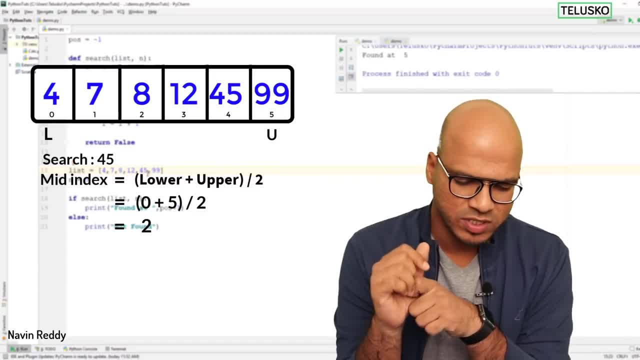 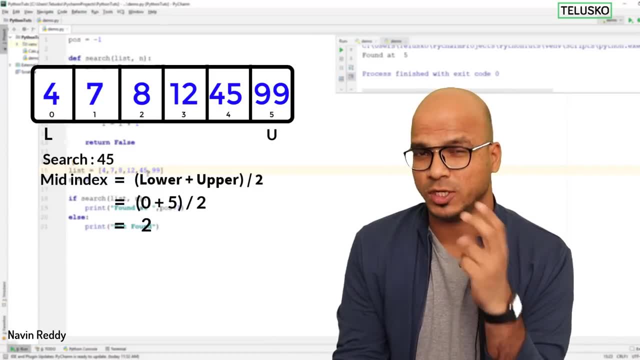 if you want to search 45 so you can see. we got the mid value right. so what's the mid value? so the index value for 4 is 0. the index value for 99 is 5, so 0 plus 5 is 5 and 5 divided by 2 is 2, right? so 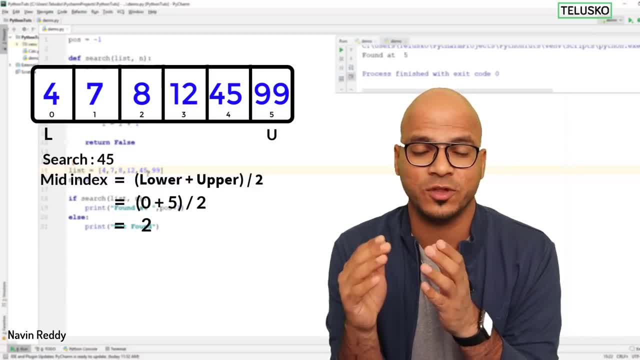 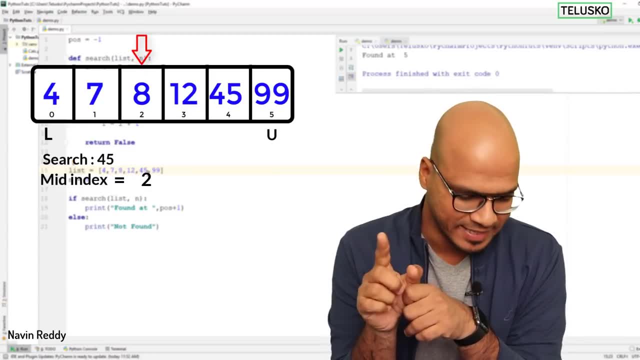 we are doing integer division here, right. we are not doing float division, so we are doing int division. so it will give you 2.. so the value at index value 2. so basically your mid is 2 now. so the value at that index is 8, right. so now we got 8 as the mid value. the next step is you have 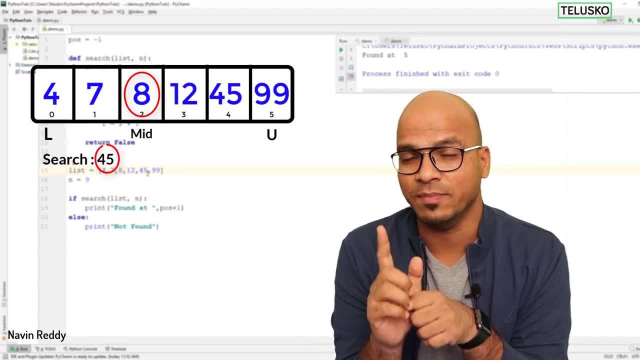 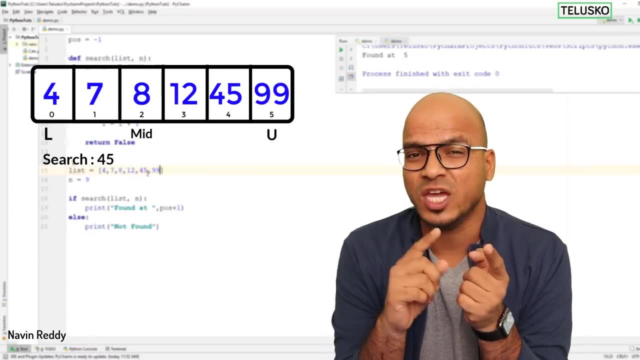 to check the mid value which you have got is matching with the element which you're searching for. the element we are searching for is 45, right, so it's not matching. now the next step would be you have to change your lower bound or upper bound. for the next iteration, you have to change your 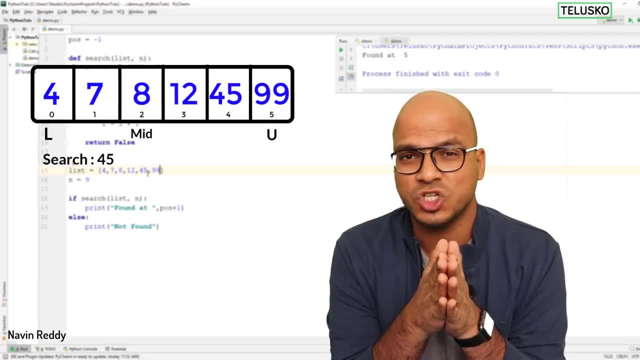 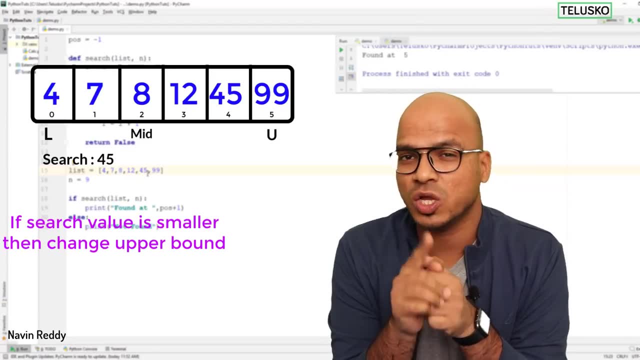 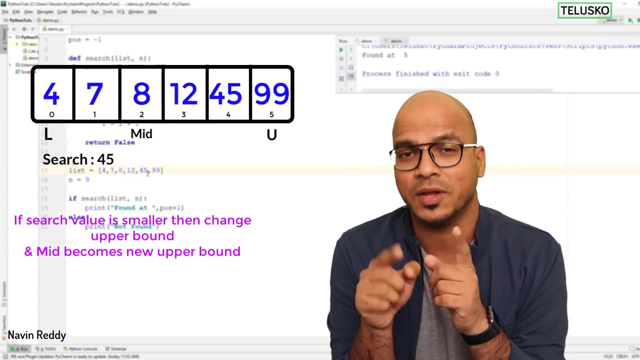 lower bound or upper bound? now which one to change? for this you have to check the value you are searching for is smaller or bigger than the mid value. if the value is smaller, change your upper bound. that means you will simply say the mid value is the new upper bound. if your value is greater, 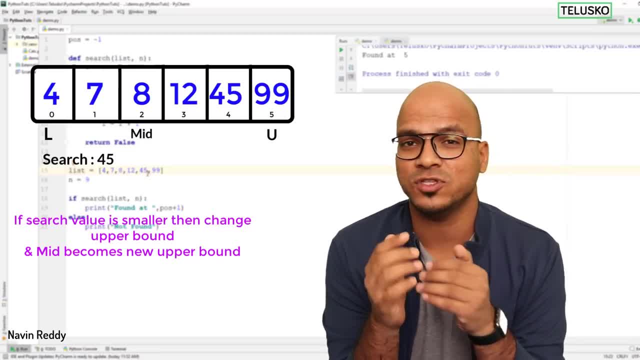 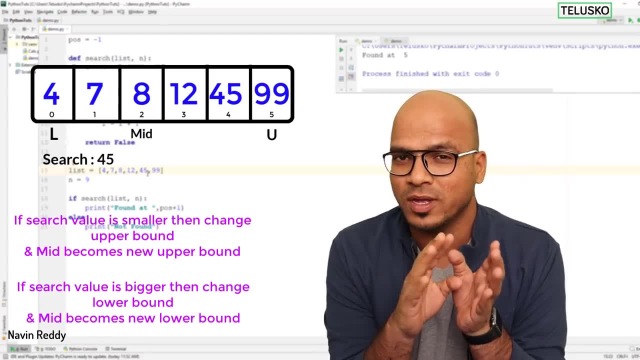 than the mid value. so the mid value here is 8, right, and the value which you're searching for is 45. so now you have to change your lower bound. so what you will do is so the old lower bound. now it will shift to the mid value, so your m becomes l, right. so instead of having a big list, now you got. 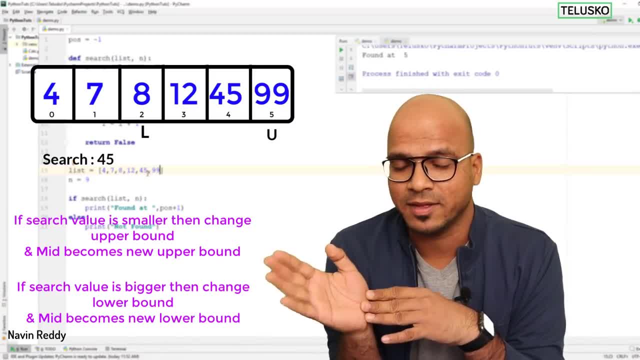 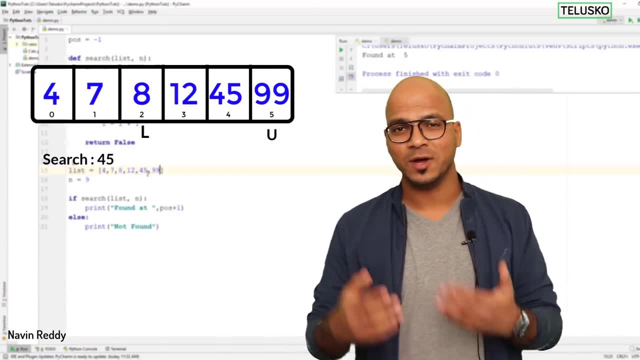 least right. so the so the least start with 8 and it ends at 99. now you got a new lower and the upper value. so what you will do, you will again find the mid value. so that's what you do every time. so your lower plus upper. so what is your lower? lower is basically 2 and your upper is 5. 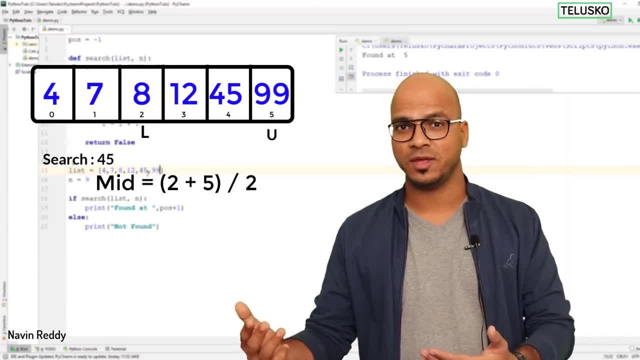 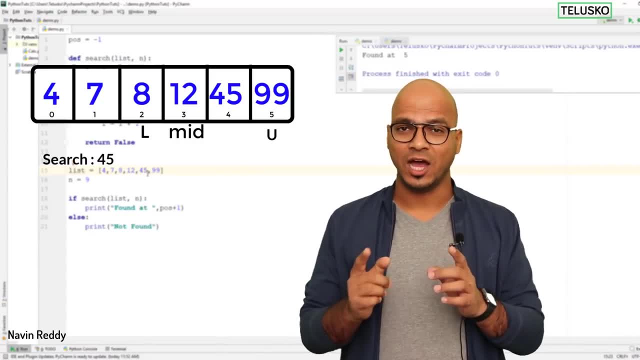 2 plus 5 is 7. 7 divided by 2 is 3, right, so now 12 becomes your new mid value. is it matching again the same thing? it's not matching right. we are searching for 45. now you have to change your. 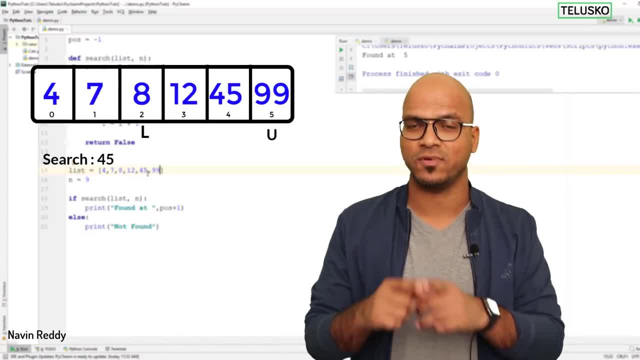 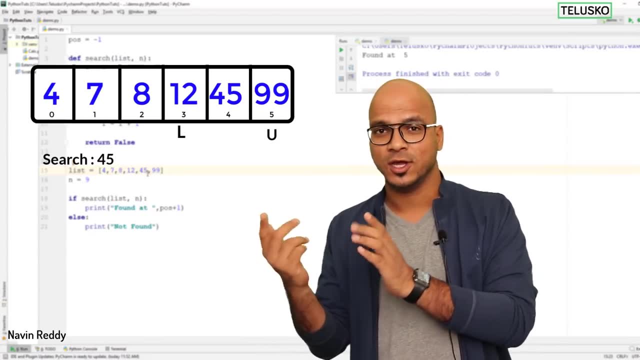 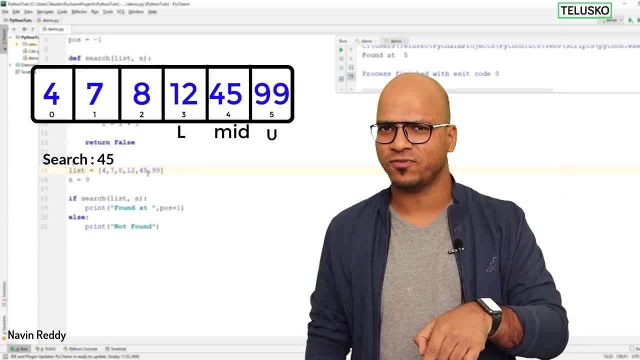 lower value again, because 45 is bigger than 12. so you will shift your lower value to 12 now. so your 12 is the lower value and 99 is upper value. so what you will do now is you will simply say mid again. the lower value is 3, the upper value is 5, so mid becomes 4, and at 4 we have 45, right so? 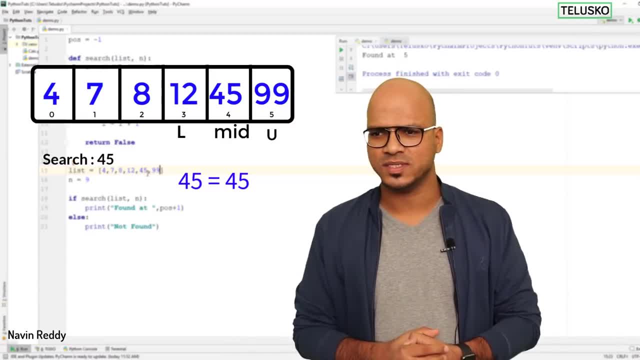 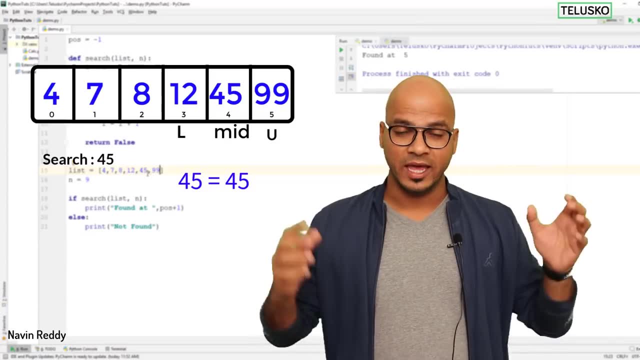 now you will check and you got the value. now you might be thinking, oh, is it a good way of doing that? and the answer is yes, because in the initial level you are skipping some values. you're not checking all the values if your list is. you're not checking all the values if your list is. 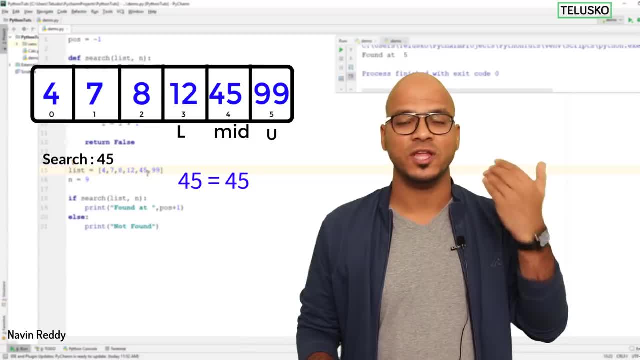 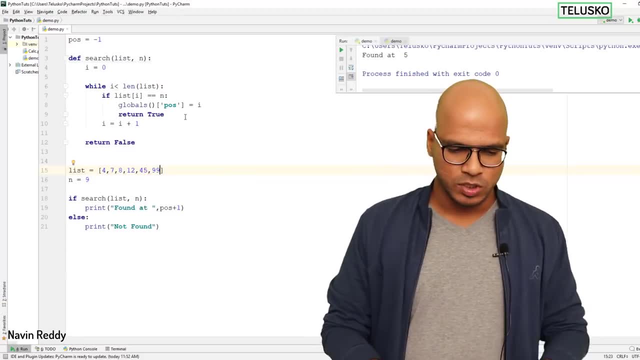 big. it will skip a lot of values which you're not checking. okay, so it will improve the speed as well. the only thing is you have to. the values which you are taking should be sorted. let's implement this with the code now. so what you're going to do is let's keep the same code we have. 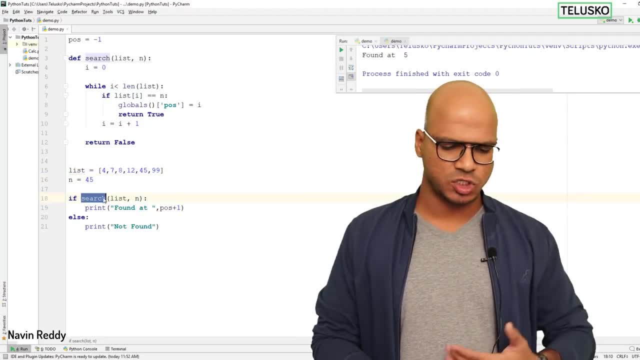 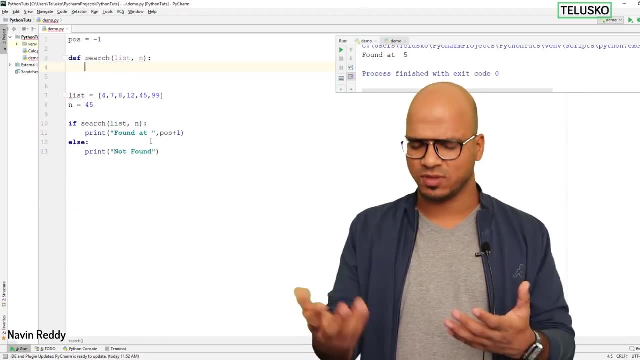 the list of values. here, let's search for 45, and so we are saying search least, we are passing the list, we are passing n, but we have to change something right. we have to change logic here, so let me just remove the entire stuff. this is something which will change right now. the first: 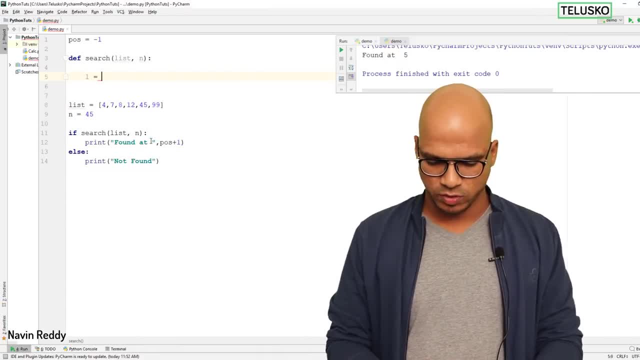 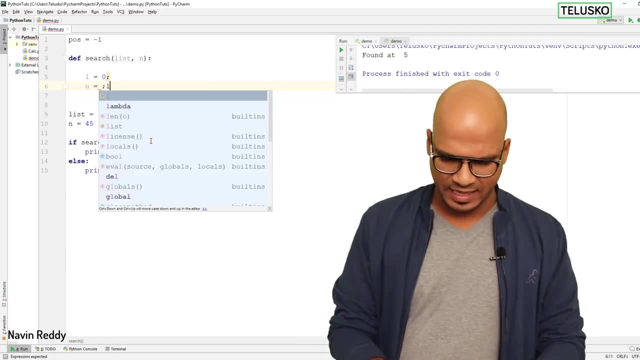 thing is you have to mention the lower bound, upper bound, right. so you will say l is equal to 0, so you will always start l with 0 and you will say u, which is the upper bound. so l is lower bound, u is upper bound. upper bound will be the length of the added right, so you will say length of the least minus 1, because 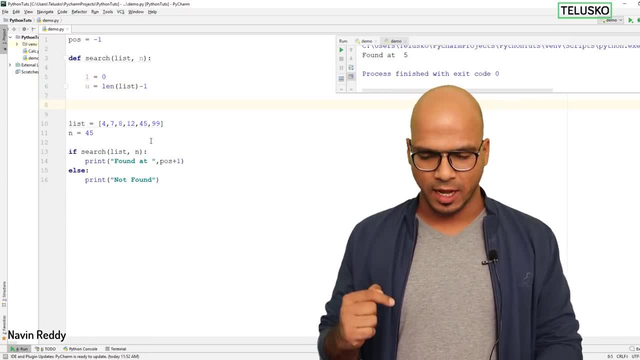 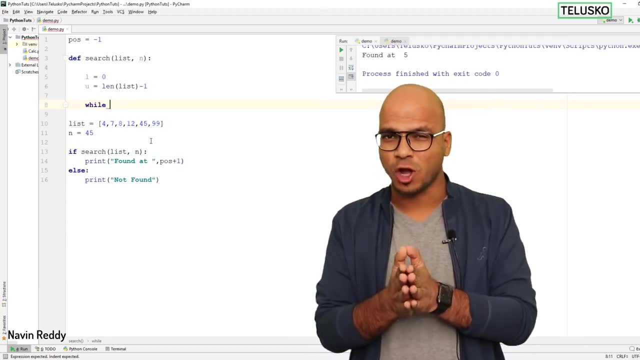 it should be 1 less than this stuff. now, once you got the lower and upper, let's apply a loop this time again. i will go with a while loop now. till what point you have to reach there? so you have to stop at two scenarios: one, the moment you found the value, and second, your lower bound should not. 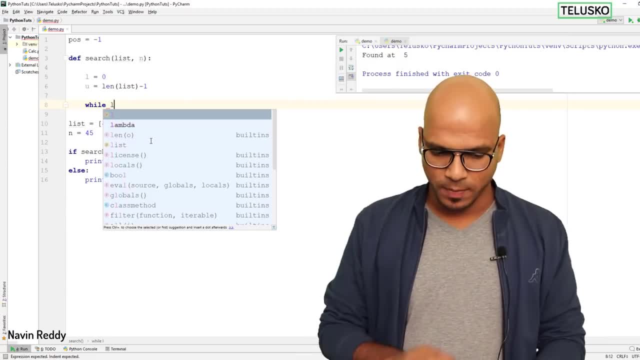 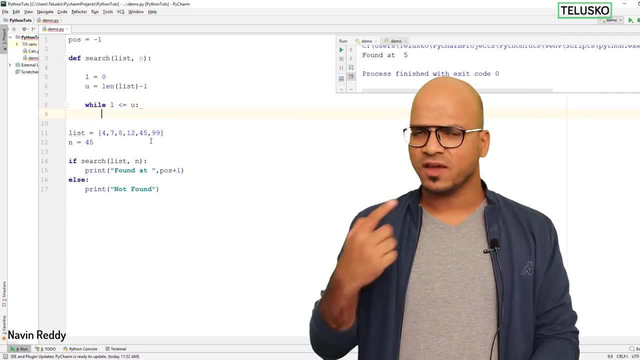 be greater than upper bound. okay, if that happens, you have to stop it. so your lower bound should be always less than or equal to the upper bound. okay, should be less than equal to. okay, should not be greater than equal to. and then you have to also stop at the. the moment you find the 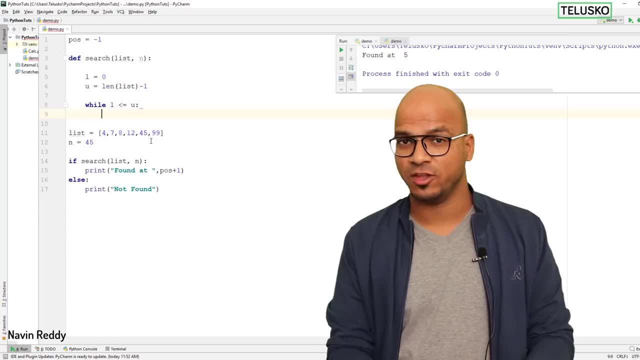 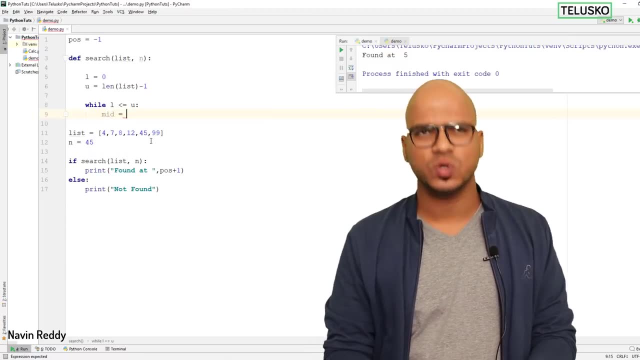 value, right, so let's do that later. so in this, while you have to, you have to find the mid-value now, right? so once we got lower, once we got upper, every time you have to find the mid value, so you will take mirror is equal to. how do you find mid it? it's lower plus upper by two, right, so you will. 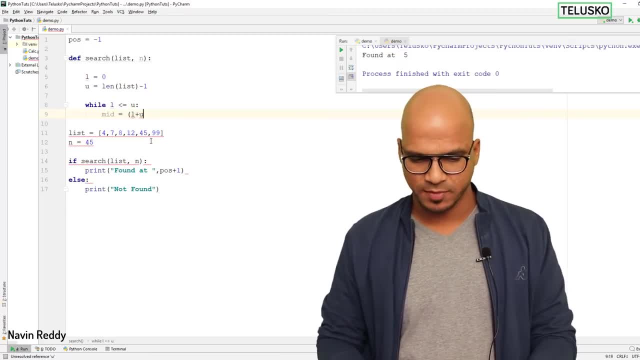 say lower plus upper, and if you say divide by two, so you will keep this in bracket. now you want a integer division, right, want a normal division. so you will use double slash, which we have done before. double slash will give you into the division and you got mid value. now you will check if the mid value so mid. 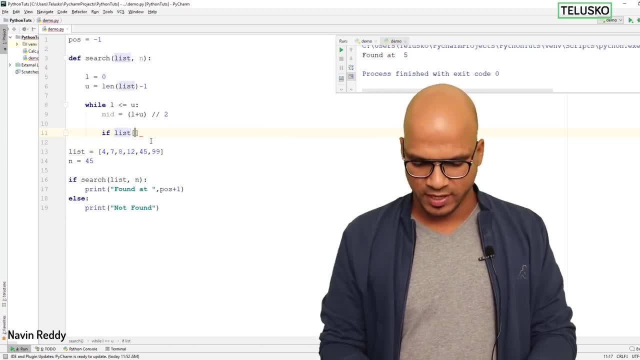 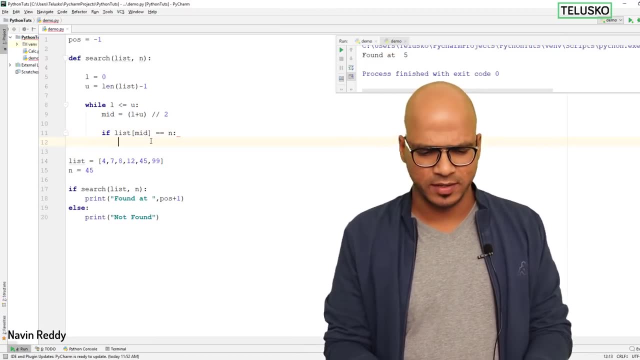 index. so we have to find the value for the mid index right, and the way you do that is by saying list of mid. if this is matching with the value which you're searching for, which is n, our job is done right. you will simply print found. in fact, i also want to mention the position right, so you 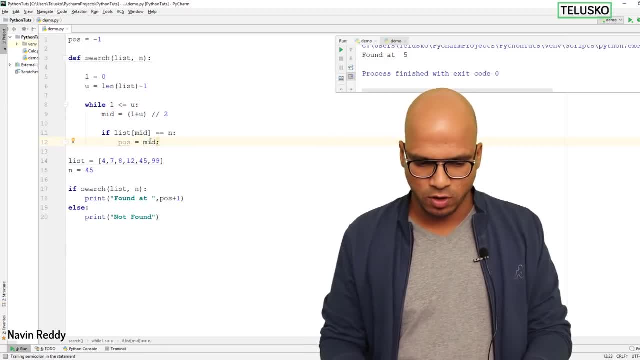 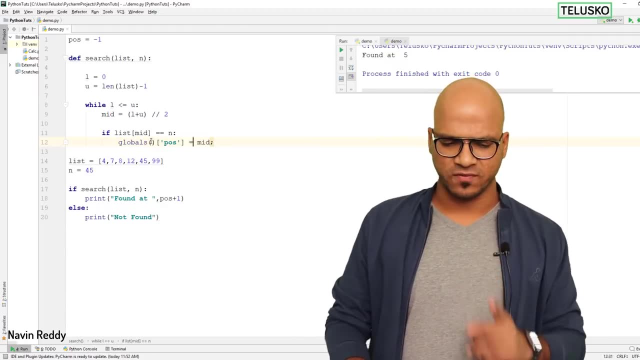 will say: pause is equal to mid, because that's the position you were looking for. oh, but pause becomes a local variable, right? so let's make it global variable. here we are saving that position as well. and then you have to do one more thing. we simply have to say: break. right, that's very important, or? 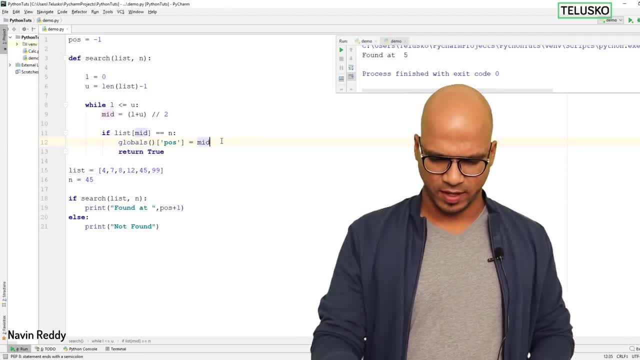 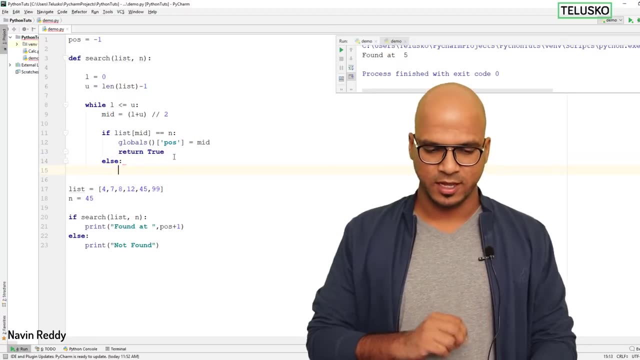 we can simply return true. why i'm using semicolon everywhere? that's it. once you got the value, you will simply return true. otherwise, what if the value is not there? so you will go for else. if the value is not matching in else, you have to do some extra stuff, which is you have to say: if now you 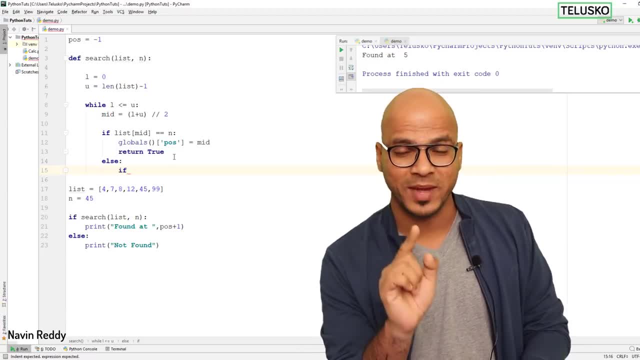 have to change your lower bound, upper bound, right, because, if you remember, if your mid value is not matching with the value which you're searching for, you have to change your mid value, which is not matching with the value which you're searching for. you have to change your lower bound or the upper bound which you want to change. depend upon the value is. 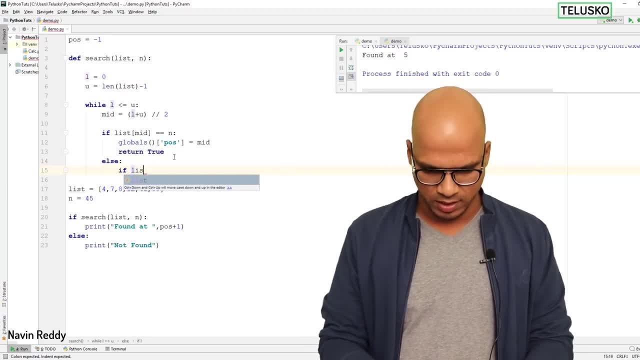 greater than the mid value or smaller than the width value. so you will check list of mid is smaller. if it is smaller than the mid value, you have to go. you have to change your upper bound right. so you will say: if that is smaller than the value which you're searching for, which is 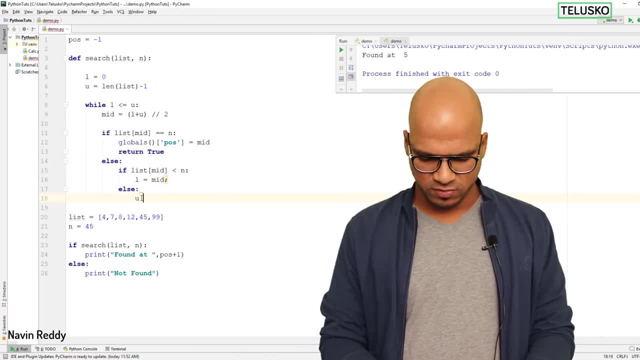 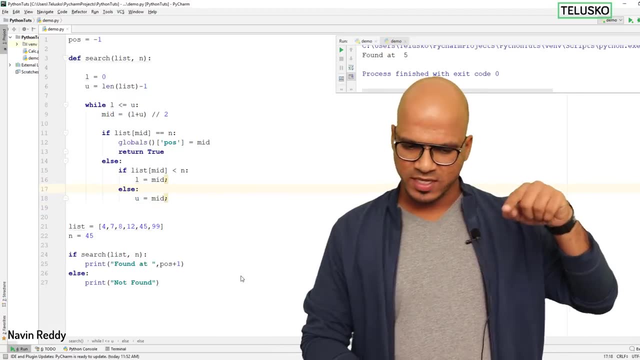 n change the lower bound and in the other case you have to change the upper bound. now let's see if that works. i feel something is wrong, but let's verify. so what i will do is i will simply run this code. it works. you can see that it says: 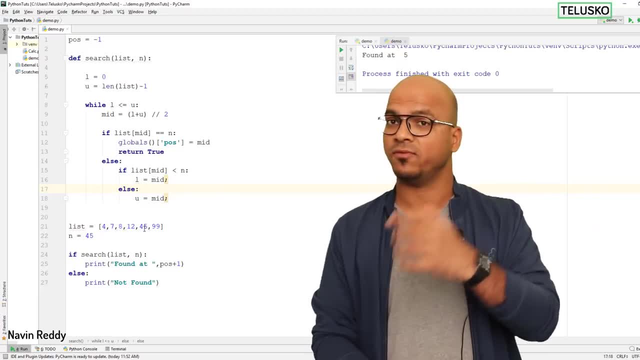 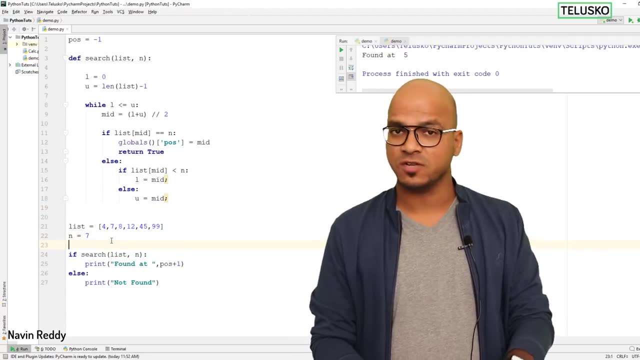 found at 5, is it right? 4, 7, 8, 12 and 5, 45, that's great, right. and let me just do it for some other value now. let's say maybe 7, and you can see if you're searching for 7, it will still work you. 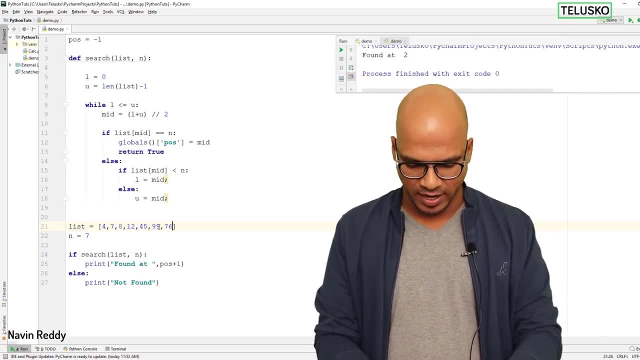 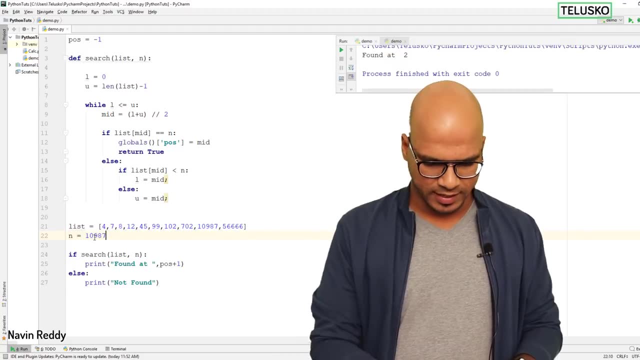 can see it says 2, and if you have a bigger list as well, let me just add some more values to here, so it doesn't matter how much, how big value you're searching for. and let me search for 10987. the moment you search for this around this, you can see it says at 9 position, is it right? 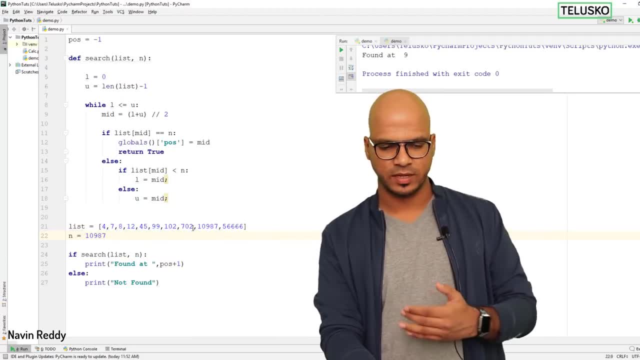 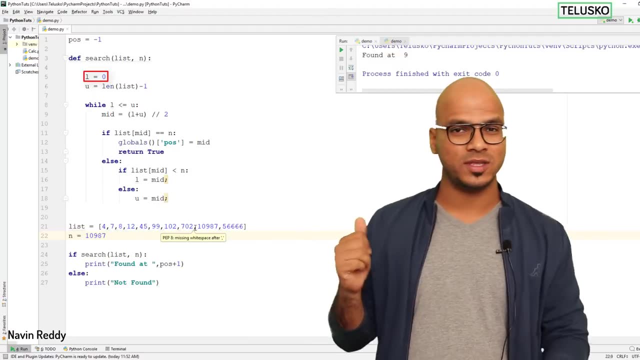 1, 2, 3, 4, 5, 6, 7, 8, 9. that's great. so this is how you do a 1-8 search. so just to repeat, just to reiterate: what we are doing here is: so we got the lower bound, we got the upper bound, and then 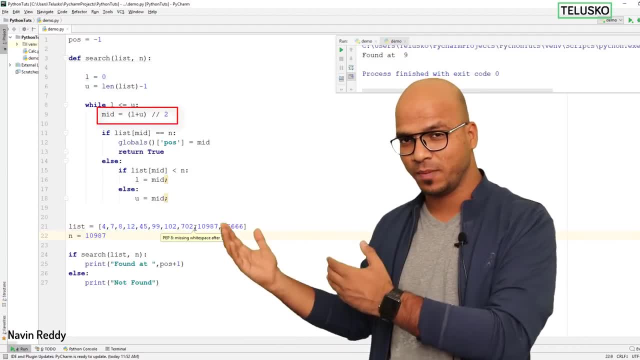 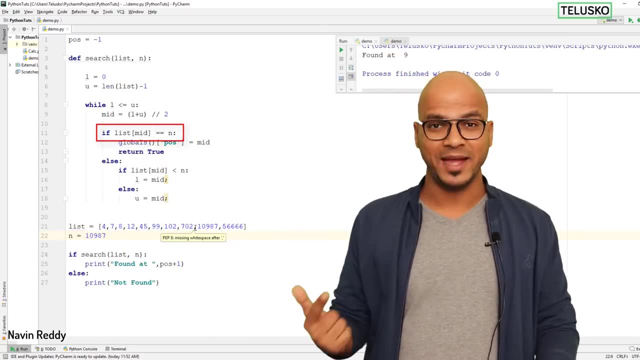 you are finding the mid value. so mid value is basically the addition of lower bound, upper bound, divided by 2. okay, now, once you've got the mid value, you have to compare that mid value with the value which you're searching for. if it is matching, that's great. so if it's not matching, 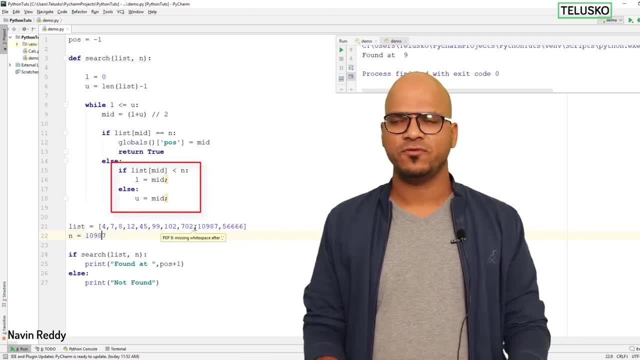 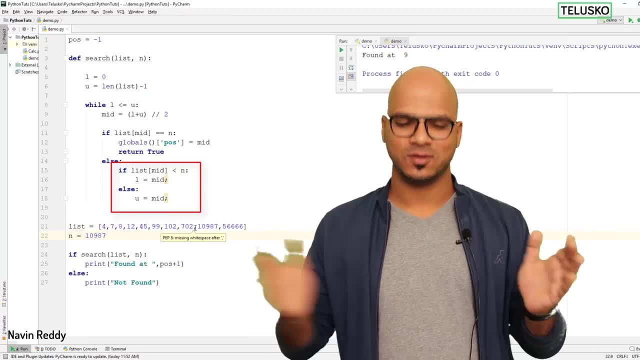 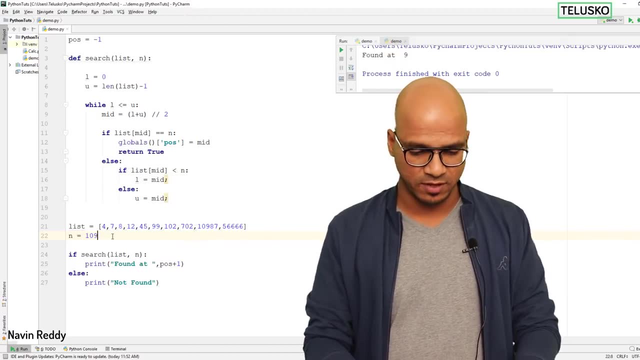 or the upper bound. so because you have to reduce the size of the array or the list, right. so depend upon, is it belongs to right hand side or left hand side, you will change it. so that's how it works, but then we have not done for something which is not there. example, if i search for 10 and